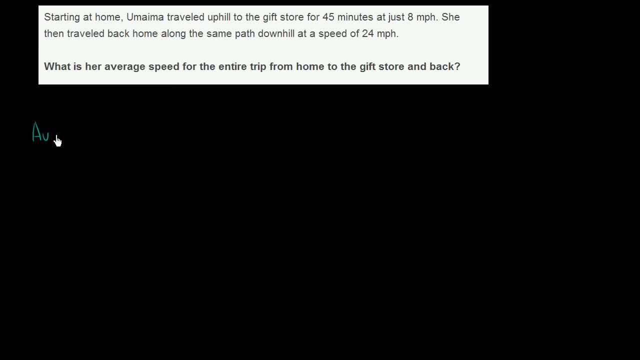 to the gift store and back. So we're trying to figure out her average speed for the entire trip. That's going to be equal to the total distance that she traveled over the total time. Well, what's the total distance going to be? 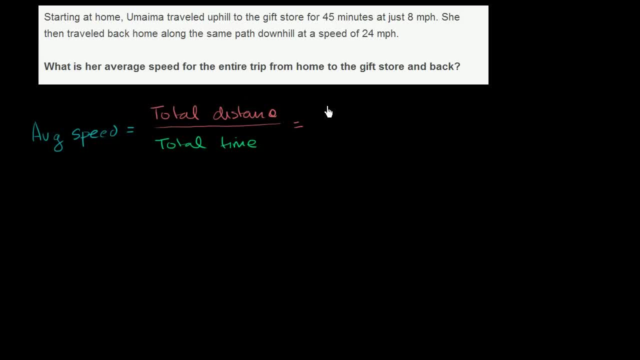 Well, the total distance is going to be the distance to the gift store and then the distance back from the gift store, which are the same distances. So it's really you could say 2 times the distance to the gift store. So 2 times the distance to the gift store. 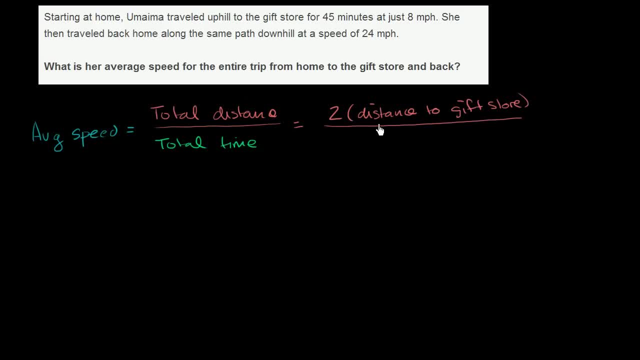 And then what is going to be her total time? Well, it's time to the gift store. So it's time to gift store, And then plus the time coming back from the gift store. Now we know that the distance to the gift store 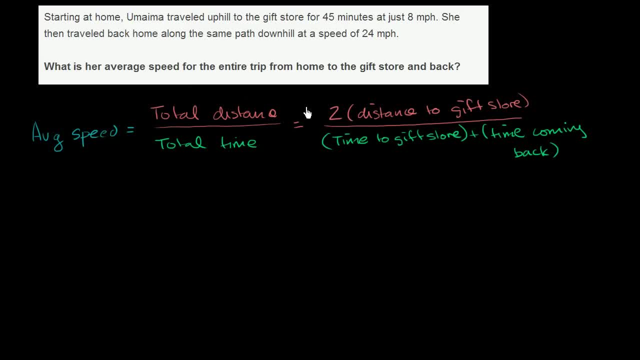 and the distance back from the gift store is the same. So that's why I just said that the total distance is just going to be 2 times the distance to the gift store. We don't know. In fact, we know we're going to have different times. 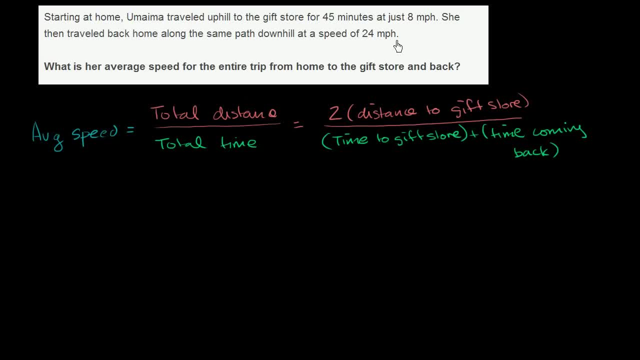 in terms of times to the gift store and times coming back. How do I know that? Well, she went at different speeds So it's going to take her. actually, she went there much slower than she came back, So it would take her longer to get there. 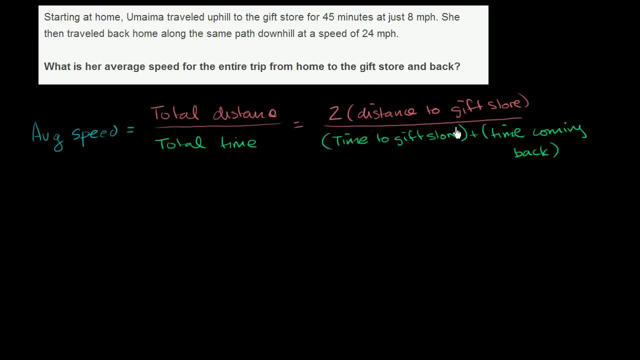 than it took her to get back. So let's see which of these we already know. So how do we figure out the distance to the gift store? No point here. do they say, hey, the gift store is this far away? But they do tell us this first sentence right over here. 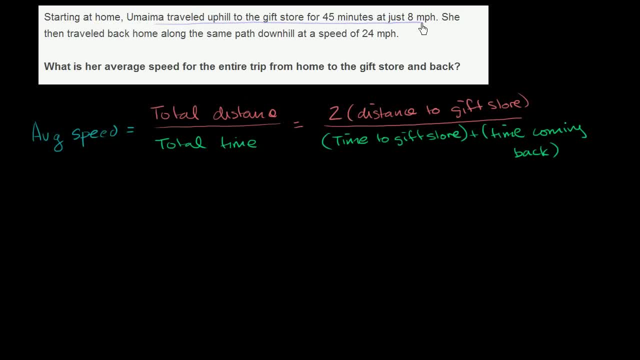 Umama traveled uphill to the gift store for 45 minutes at just 8 miles per hour. So we're given a time and we're given a speed. We should be able to figure out a distance. So let's just do a little bit of a side here. 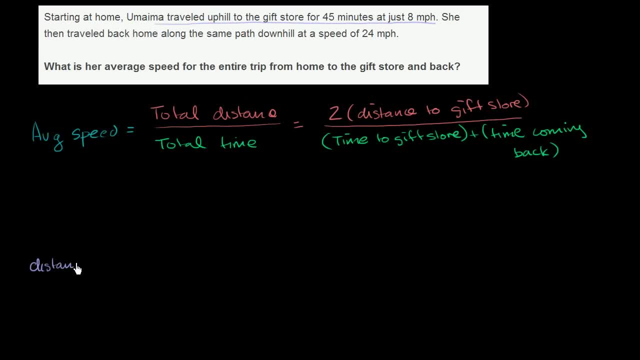 We should be able to figure out the distance to the store. Let me write it this way: Distance to the store. Distance to store will be equal to- and we've got to make sure we have our units right Here. they gave it in minutes. 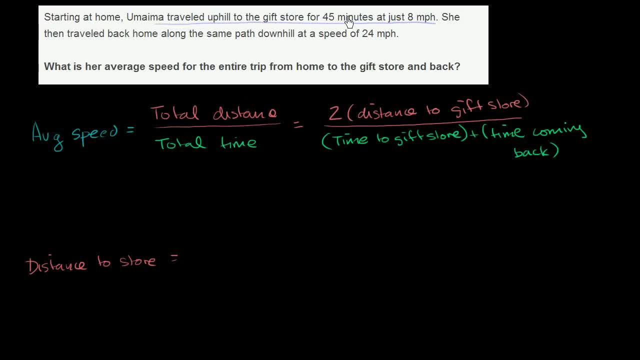 Here they have 8 miles per hour, So let's convert this into hours. So 45 minutes in hours, So it's 45 minutes out of 60 minutes per hour. So that's going to give us 45 sixtieths. 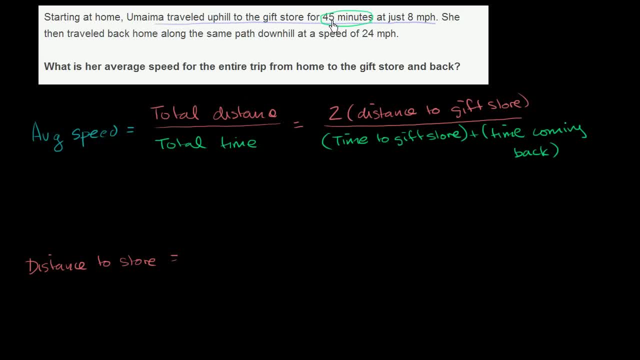 Divide both by 15.. That's the same thing As 3 fourths, So it's going to be 3 fourths hours. 3 fourths hours is the time. Times: an average speed of 8 miles per hour. Times: 8 miles per hour. 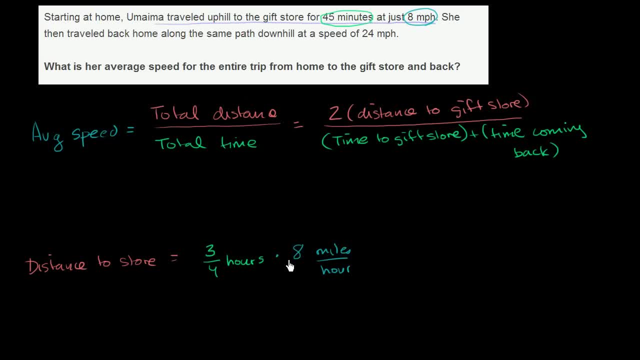 So what is the distance to the store? Well, 3 fourths times 8, or you could do it as 3 fourths times 8 times 1, is going to be 24 over 4.. Let me just write that. 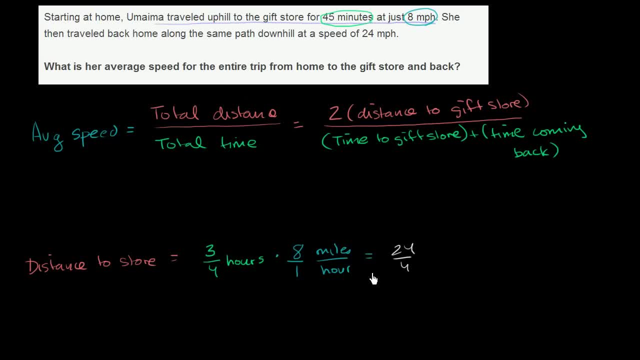 That's going to be 24.. 24 over 4, which is equal to 6.. And units-wise we're just left with miles. So the distance to the store is 6 miles, 2 times the distance to the gift store. 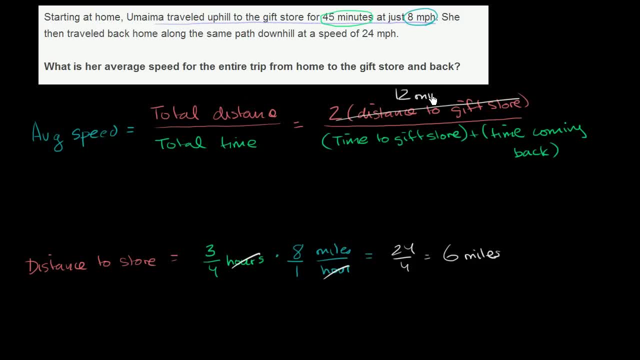 Well, this whole thing is going to be 12 miles. 12 miles is the total distance she traveled. Now, what is the time to the gift store? Well, they already told that to us. They already told us that it's 45.. 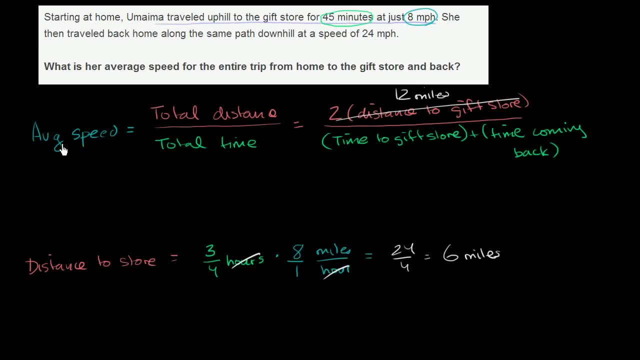 45 minutes. Now I want to put everything in hours. I'm assuming that they want our average speed in hours, So I'm going to put everything in hours. So the time to the gift store was 3 fourths of an hour. 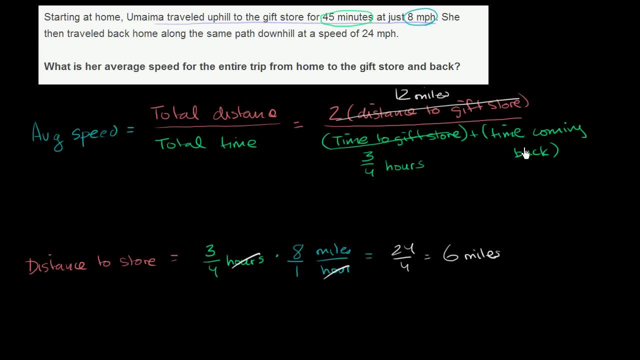 3, fourths hours, And what's the time coming back from the gift store? Well, we know her speed. We know her speed coming back. We already know the distance from the gift store. It's the same as the distance to the gift store. 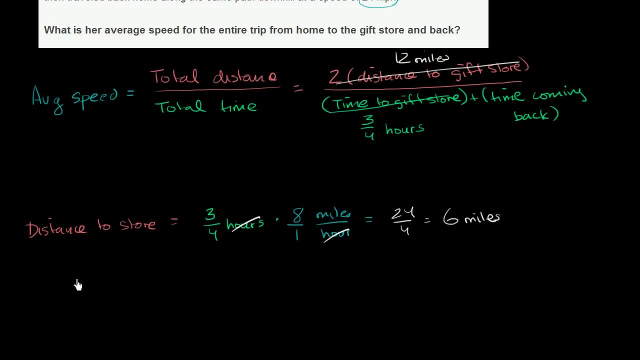 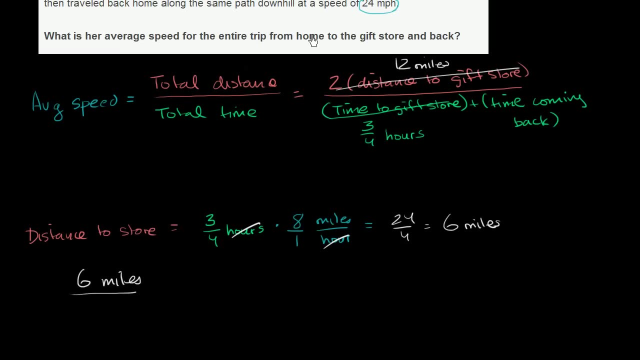 So we can take this distance. We can take 6 miles. That's the distance to the gift store. 6 miles divided by her speed coming back, which is 24 miles per hour. So divided by 24 miles per hour gives us- let's see- 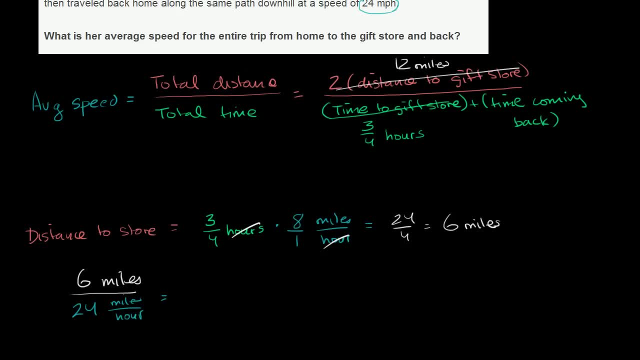 We're going to have 6 over 24 is the same thing as 1 fourth. It's going to be 1 fourth. And then miles divided by miles per hour is the same thing as miles times. hours per mile. The miles cancel out and you'll have 1 fourth of an hour.